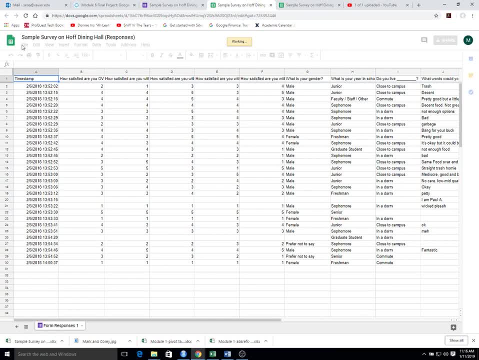 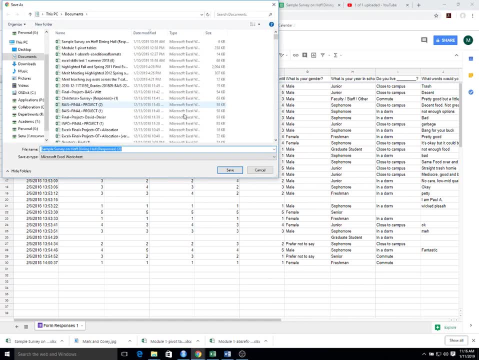 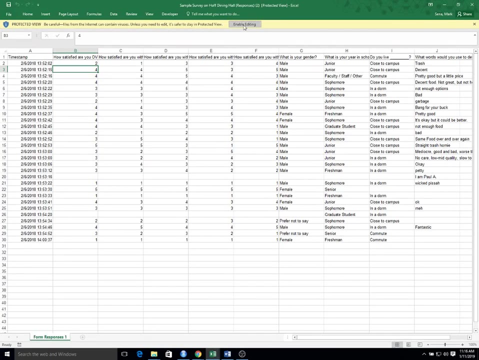 Google worksheet by clicking that green icon and I'm going to save my file, or download my file in an Excel format. So now I'm going to save and open in Excel. I'm going to enable the editing, the very first thing I'm going to do. this is very important because it 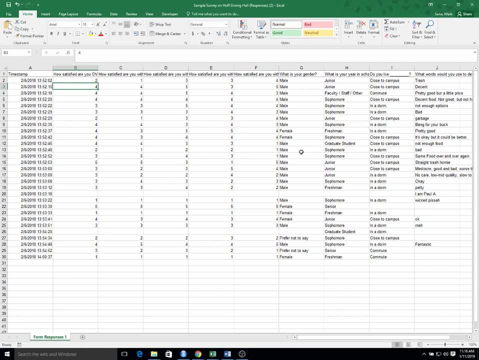 affects the, the appearance of all the things you're going to do later. so by default, Google includes the entire question as the heading on the on the datasheet, so we want to go up here to this first. that would take up a lot of unnecessary space and make things a little funny looking. so typically when 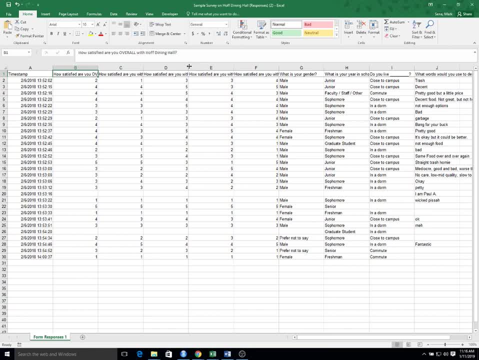 you see a chart you don't see, like, how old are you? it says age. so, for example, some labels: we typically use abbreviated labels as headings and data sets rather than long drawn-out questions. so I'm going to go into this first row and I'm going to replace 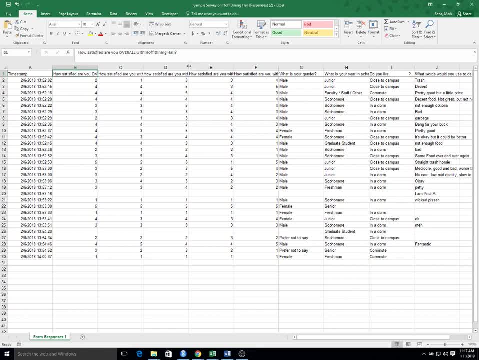 each of the the first row entries with abbreviated labels, so I'm going to try to make them all, maybe one or two words, for example, so we'll give this one as a standard. So I'm selecting the entire row, right-clicking and deleting If you have any. I didn't really have any questions where a lot of people answered things freeform that I want to. let's say, you ask somebody their major, you might want to do a sort by that and then kind of manually clean up the responses that are supposed to be the same. 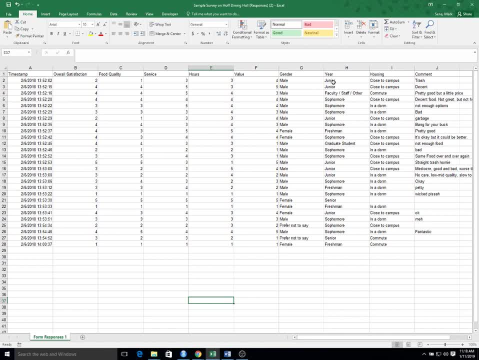 So if I had a column called major and one person put marketing and another person put MKTG, you might try to make those all the same. So just so they can be combined in any sort of analysis. But anyway, from this point we have a data set that we're. I don't do anything with the timestamp, but it's not hurting anything. 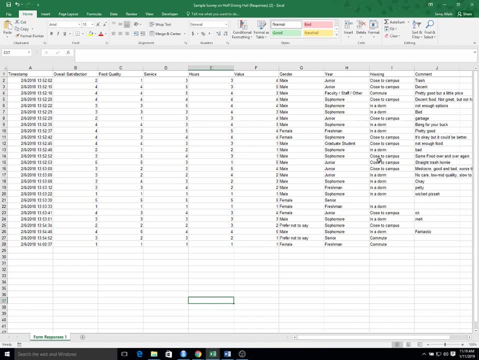 So now I have a data set and I'm ready to begin doing the analysis. So at this point the instructions are pretty similar to what we had in module one with the pivot tables, And each person's analysis is going to be different than mine because you ask different questions. 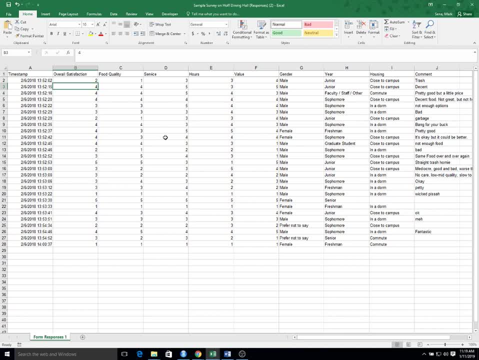 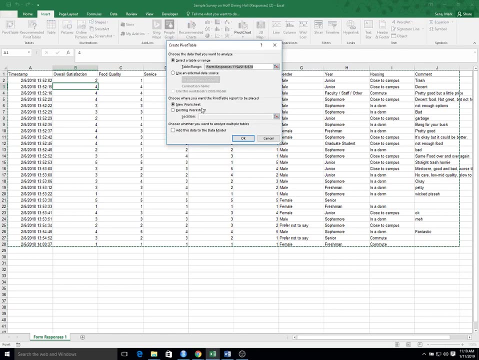 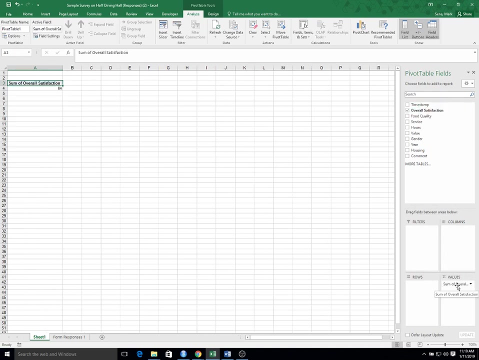 You had a different topic, But in this particular survey I'm going to start off by doing a few pivot tables just to get you started on the demonstration. So I'm going to click insert- pivot table on a new worksheet And in the pivot table I'm going to put the overall satisfaction and the sum value. 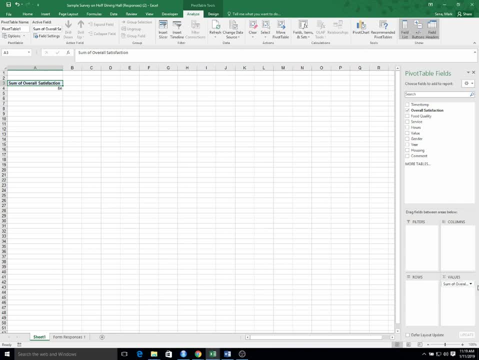 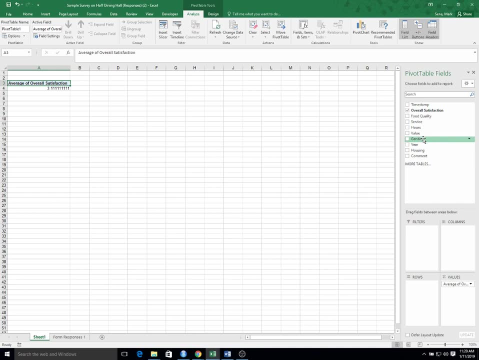 I'm going pretty fast here, because we've already done this before. I'm going to change this from a sum to an average, And then I'm going to put gender in the row. I'm going to do a little bit of cleanup here. 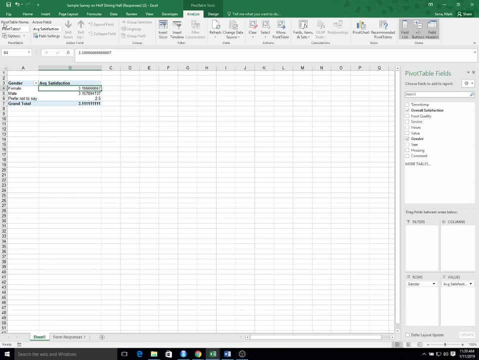 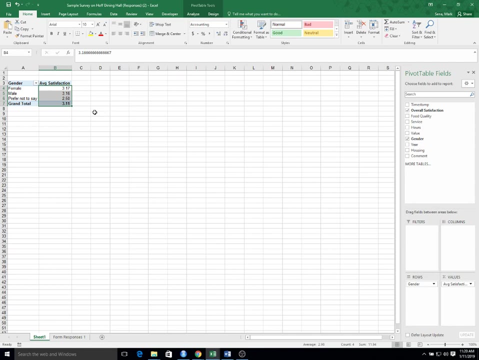 One thing I always do is format my cells and headings. So this makes it look a lot, lot, a lot nicer when you, when you do a little, just a little bit of formatting. So once I- so now I can see that there's really no difference between the males and the females. 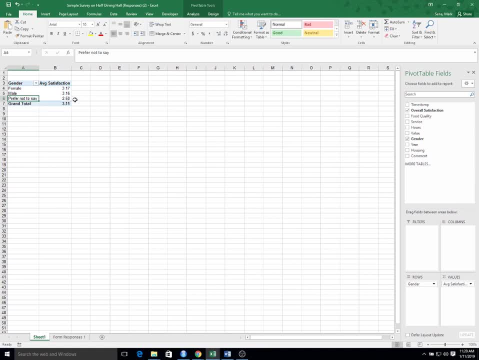 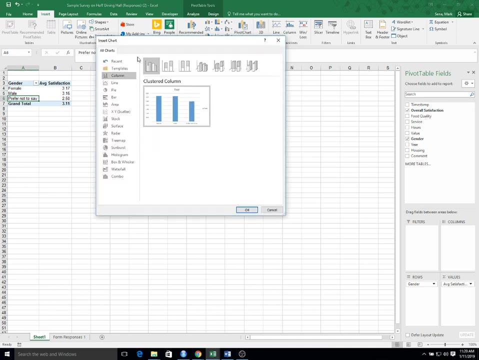 I had maybe one person that Didn't want to reveal their gender, or a couple of people, So now I'm going to also insert a chart to go along with it. So I'm going to select this pivot chart And for this one I'll just pick a, a column chart. 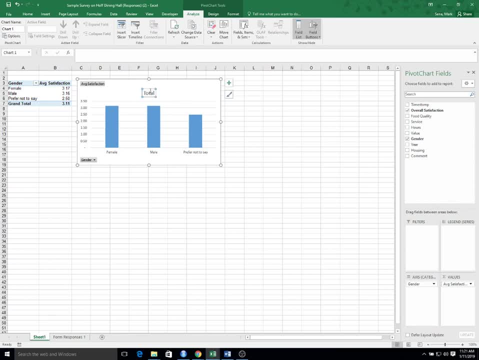 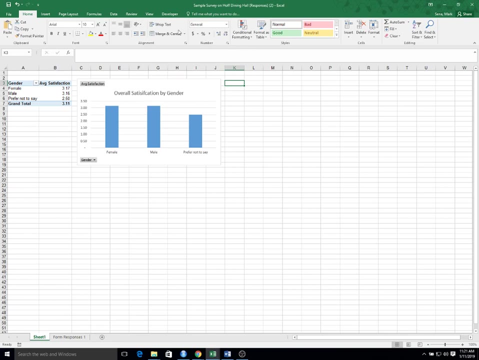 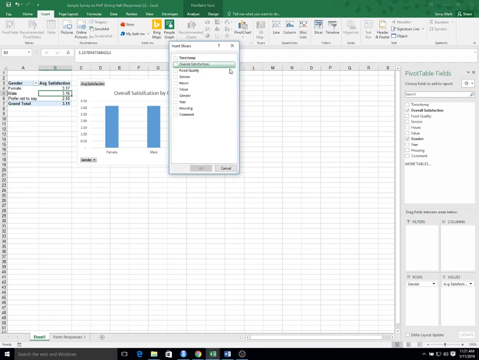 I always get rid of this total And put a meaningful label on it, And then I could also put some slicers in. So I'm going to insert slicers for the anything that I want, but mostly the demographics, like the year and the housing. 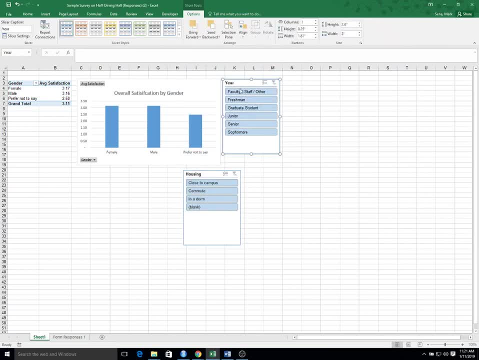 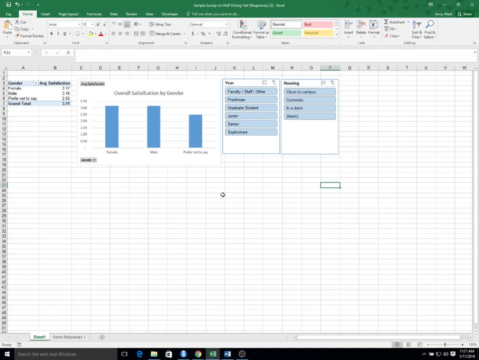 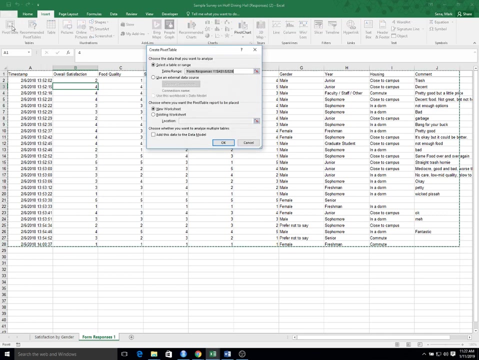 So they can see combinations And I'll give the sheet a name. Um, if I wanted to, I could make a second pivot table That's very similar. Let's say, I want to put it in the same worksheet except below. I'll request to begin right there. 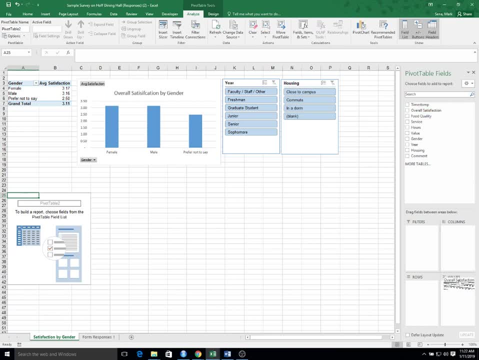 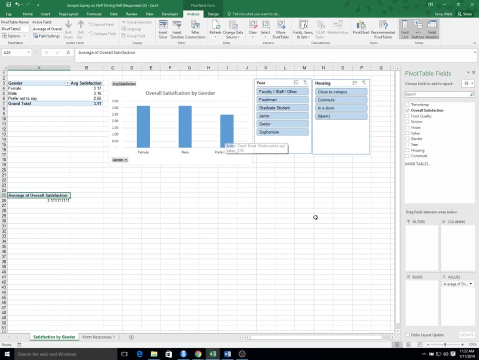 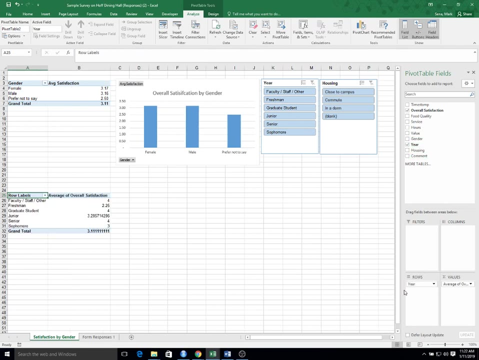 So I'm just going to do the same thing again, where I'm going to put overall satisfaction and I'm going to change it to an average, And then I'm going to copy that. So that's three, That's four, That's five. 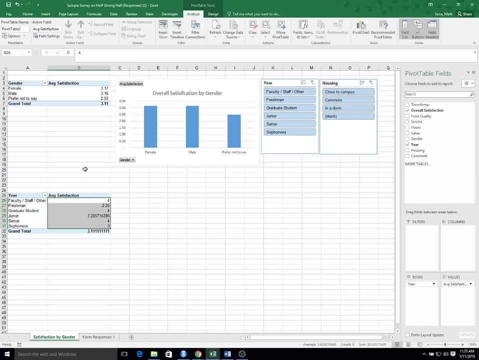 That's six, And this time, instead of putting gender in the row, I'm going to put here in the row, And of course I want to apply my formats again And again. I'm just going to enable it to run here. 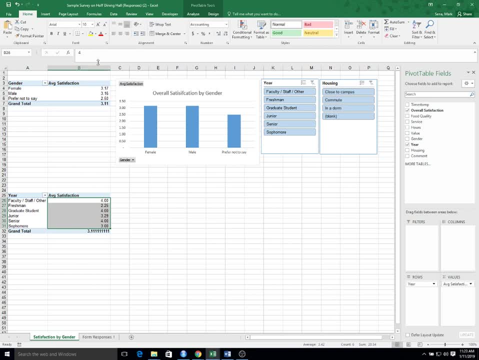 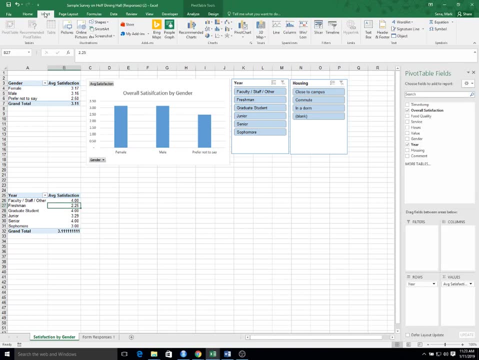 And this time, instead of putting gender in the row, I'm going to put it in the row. And this time, instead of putting gender in the row, I'm going to have this one, a particular piece of character, And again I could insert a chart. 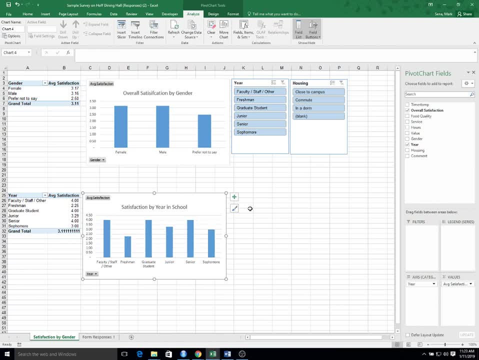 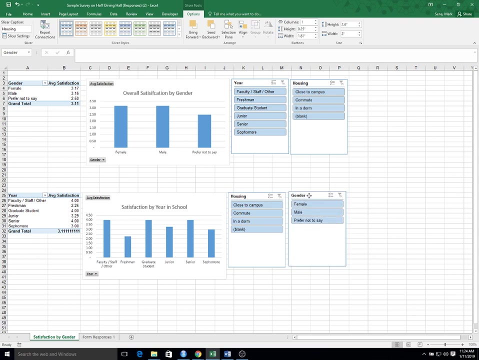 That total legend is my pet peeve. I can't stand seeing those, And I could insert slicers again. Since we already have year, this time we could put gender and housing And maybe to distinguish this one from the other one I might distinguish. 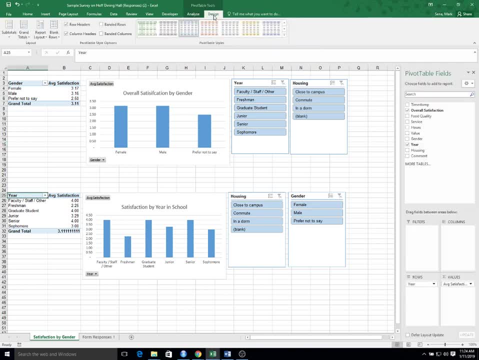 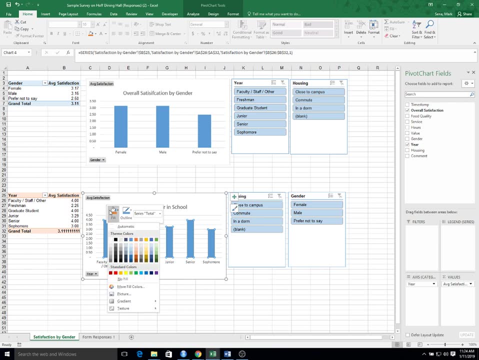 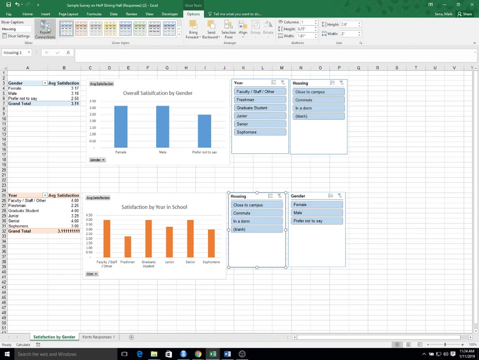 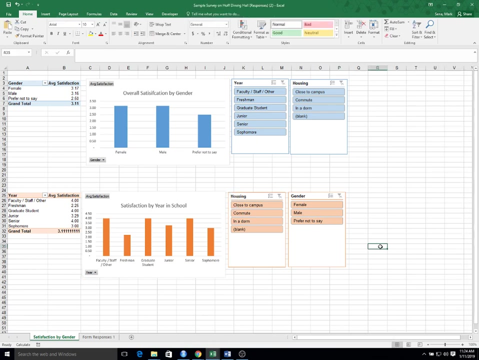 I might design this one a little bit differently by making things a different color. Okay, so that's not a thing of beauty, but you can see how I'm trying to design this one a little bit differently and how it looks halfway decent And the slicer should work. 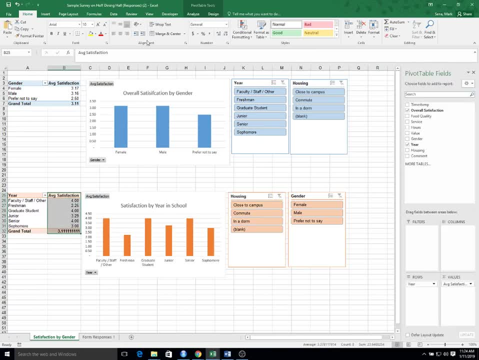 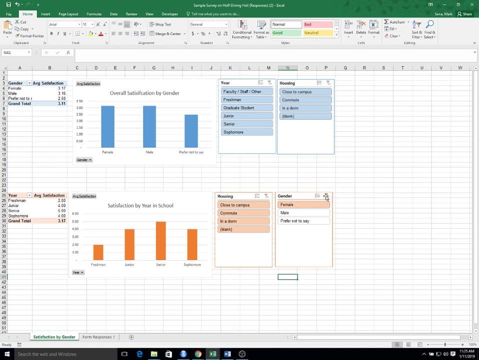 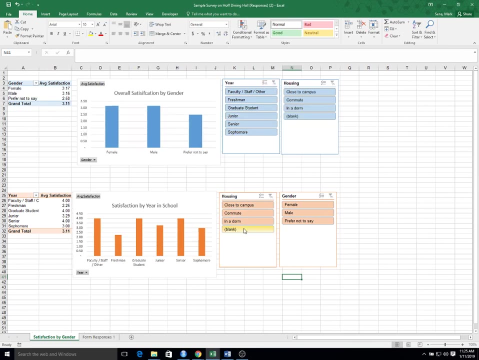 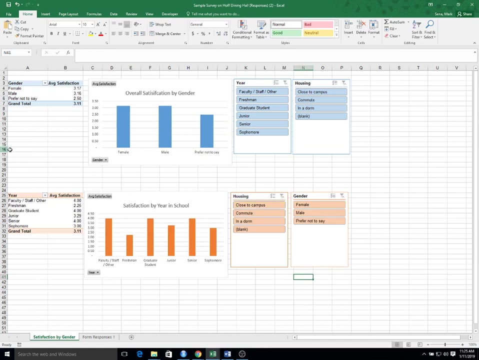 I have to make sure I have the grand total summarized as well. So I want to click the slicers to just kind of look at my data a little bit, Okay, Anyway. so looking at the data you can see that we probably didn't have a lot of seniors taking. 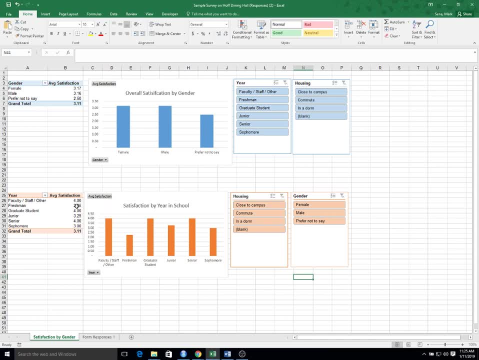 or graduate students or faculty staff taking it, but freshmen seemed a little less satisfied than sophomores and juniors, at least among the data that I collected. So let's look at a different. let's say you have some text data, So I'm going to. 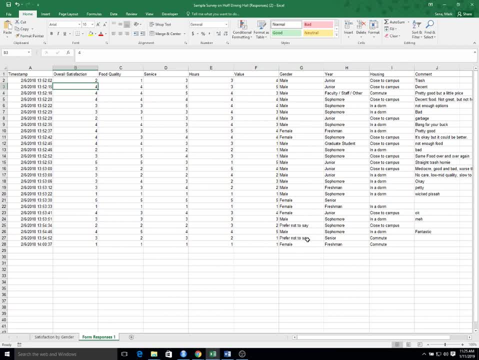 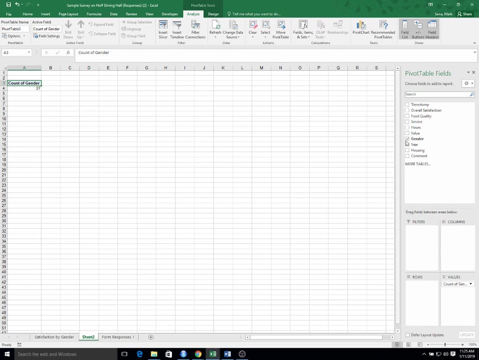 let's say I want to show the breakouts, the breakdown of the gender, just to see who took my survey. So I'm going to insert a pivot table on a new worksheet. This time I'm going to put gender in, both the sum value and in the row. 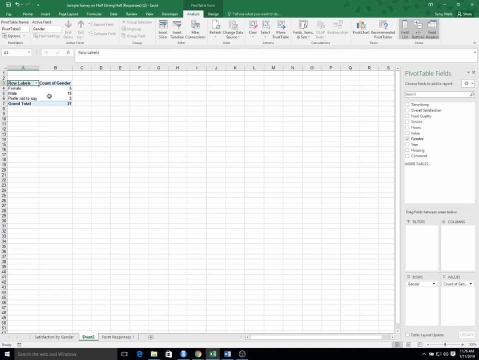 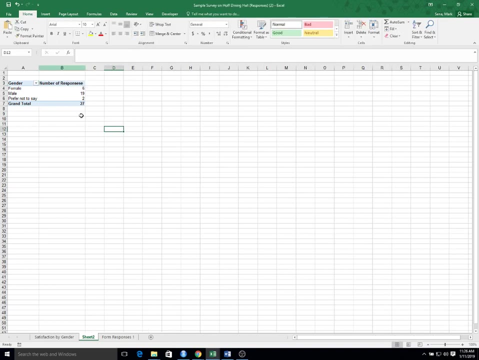 and that'll give me a count. Okay, So I'm going to put gender in, both the sum value and in the row, and that'll give me a count. So now I see how many people took the survey. I had 19 males. 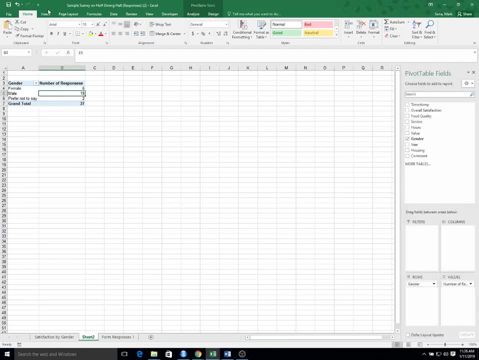 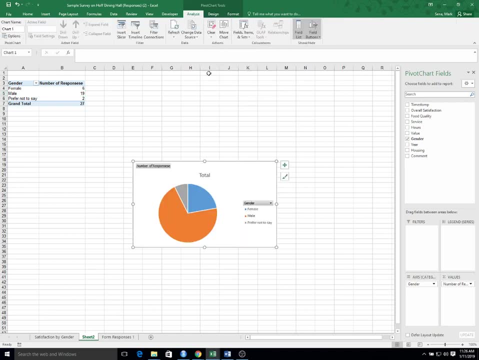 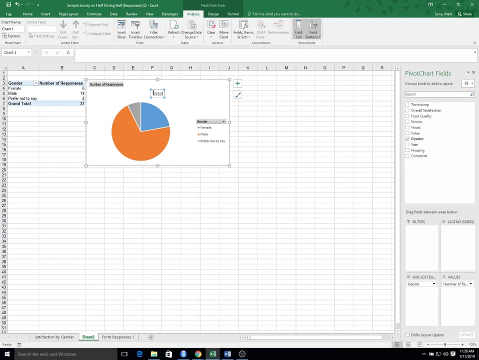 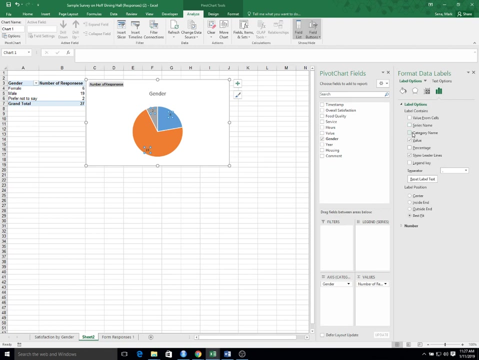 six females and two prefer not to say So. now I could insert a pie chart. I know I did this again in module one. I like to add data labels and then I like to format the data labels over here to show the category name and the percentage. 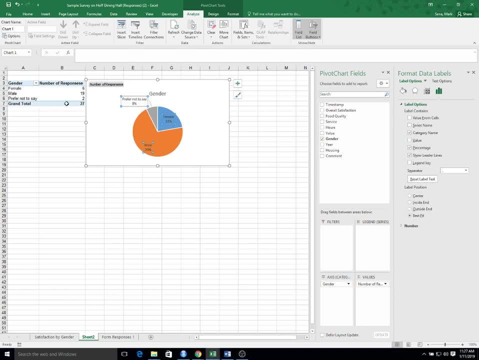 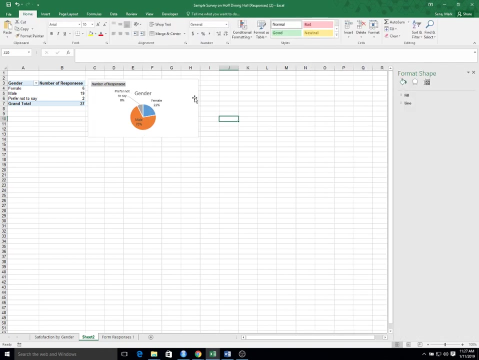 but not the value. We already have the value in the table. So by uh formatting our chart like this, we're able to kind of give some different information that's shown, that isn't shown in the table as well, And that's not too nice looking. 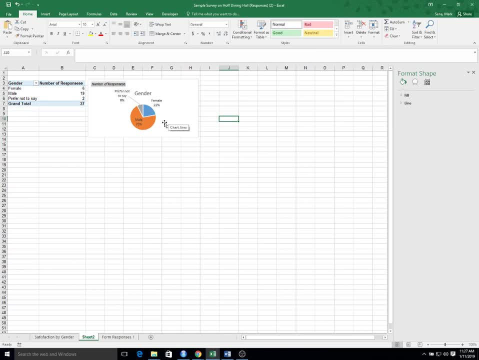 but it does. That's not too nice looking, but it does. It does the job. It's nice when you don't have a long label so everything can kind of fit in the pie slices, But anyway, you could do something similar for housing. 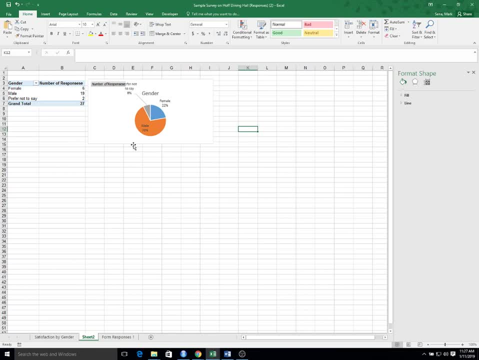 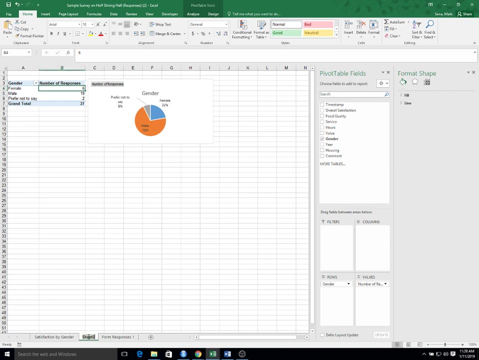 um year in school, that kind of thing, and put it in the same chart. Now you could also have slicers here, Okay, So I'm going to call this, uh, demographics And um, if I were completing this, 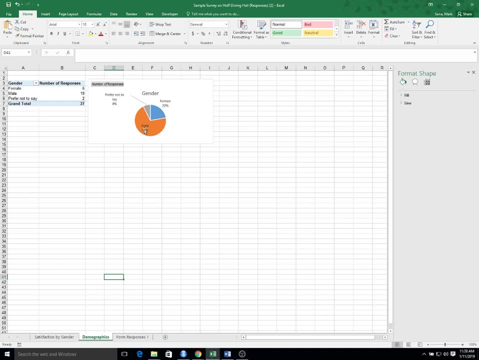 I'm not going to bore you with um doing everything repeatedly, But, um, if I wanted to, I would have maybe three of these on the same sheet. Um, I'll post a? um, a completed link as well, to a. 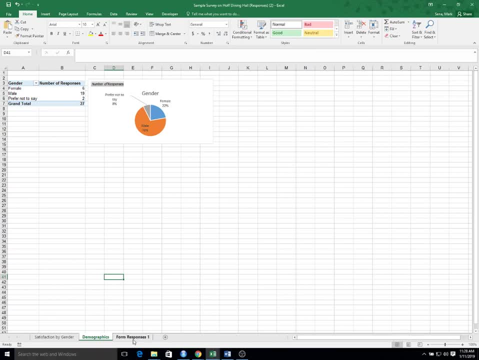 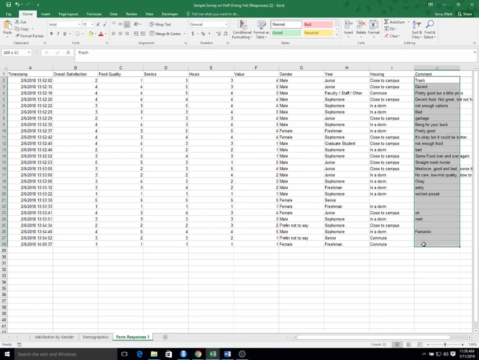 uh, a file that is done. So let me show you one more thing, Let's say on the, or two more things. Let's say I wanted to do something with these comments, So I'm just going to um, insert another pivot table. 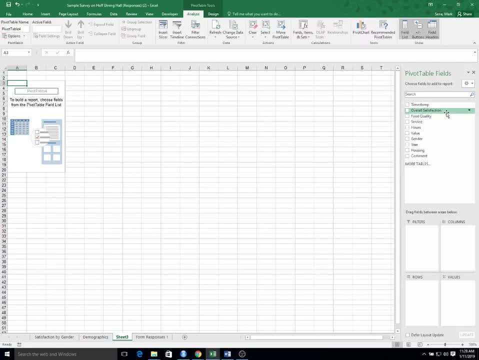 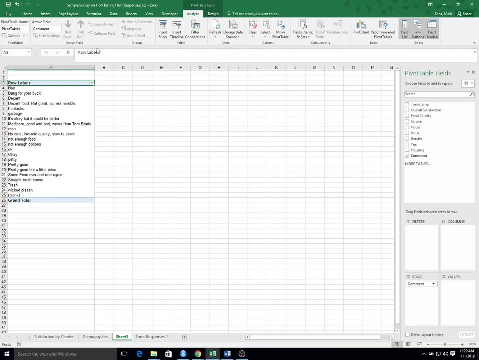 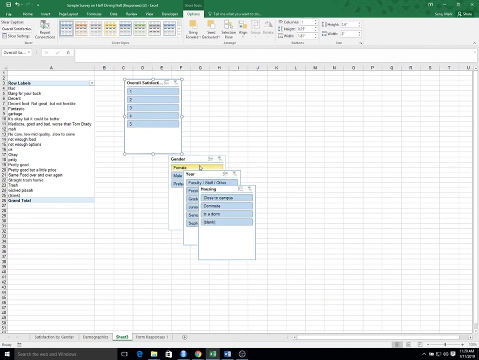 in a new worksheet And I'm going to put those comments in the row. Now we just see a list of them, And now I'm going to put a slicer in A set of slicers. So now, um, this gives the user a way to kind of interactively view the comments. 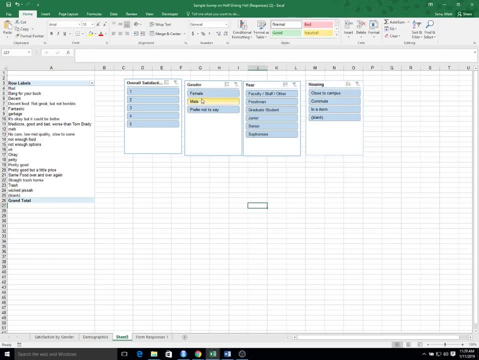 So you can see all the comments, but let's see the male comments versus the female comments. Um, or let's see the comments of those comments, of those that were unsatisfied versus those that were satisfied. Oh, that one didn't make sense. 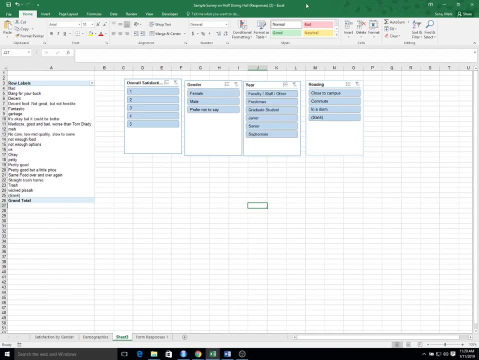 But anyway, um, hopefully you'll have better data than I had, So that's a quick way to get your comments and make them into something kind of interactive and cool. Um, and in the raw data, you can do some simple things. 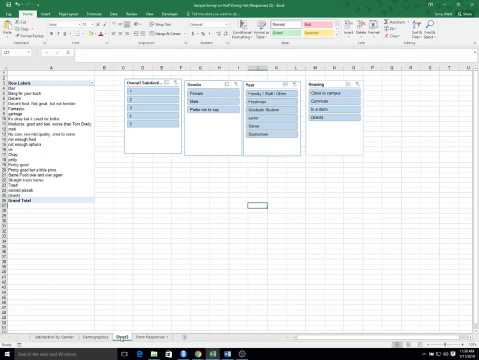 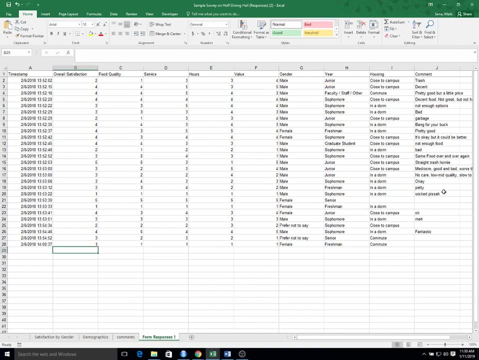 Whoops Call it comments. In the raw data you can do simple things like averages And then, once you have the uh averages, you can make a simple chart out of those, just by selecting these labels and these labels and making a bar chart out of it. 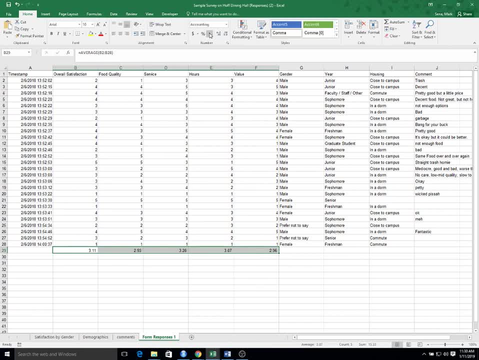 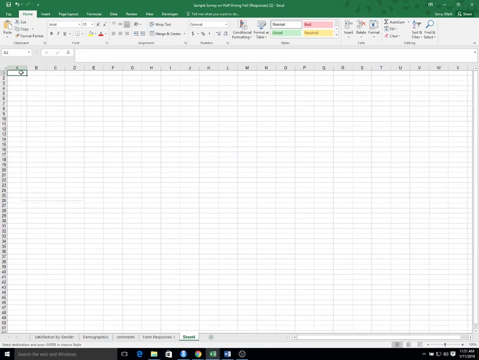 I sometimes like to uh move the data to a new worksheet And if you wanted to do a simple chart, you could um move these over. I'm going to copy the labels, go to a new worksheet and paste. 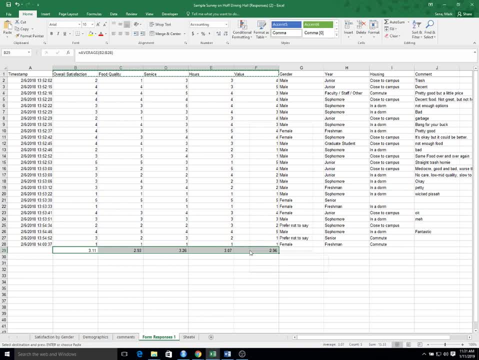 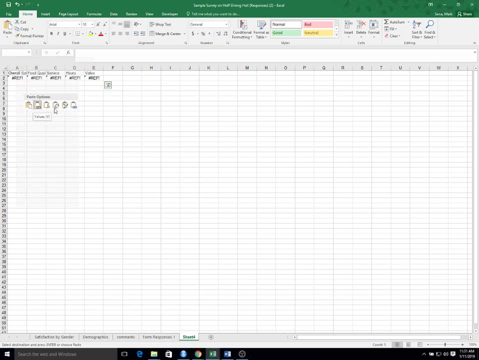 And then I'm going to do the same thing with these, Um, I'm going to paste the values for these And then, if I wanted to, I could do a copy and then a paste special. and where is the transpose? The transpose here: 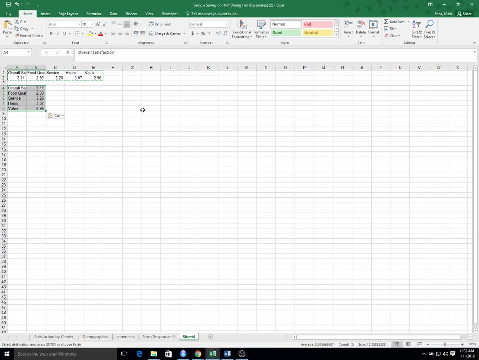 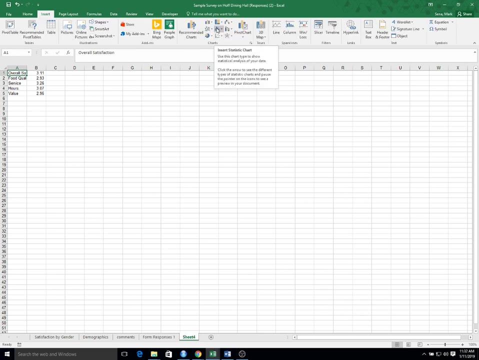 I like that. Um, and then I can just remove the original data. here I'm going to delete the cells And from here I can just insert a kind of a traditional chart. Oops, I need to select the data first. 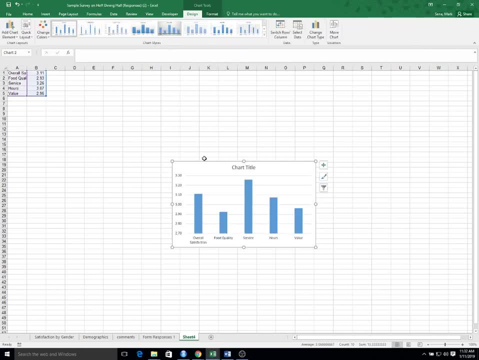 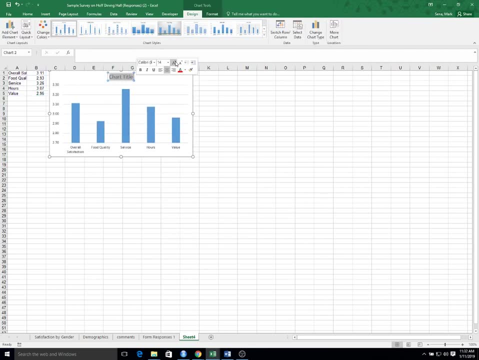 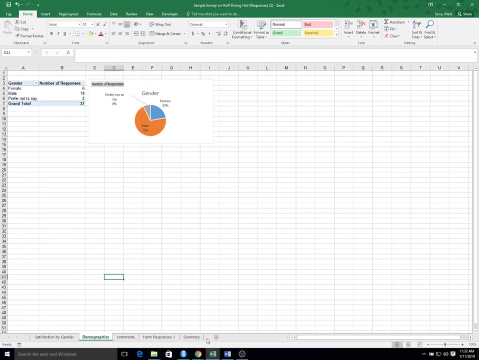 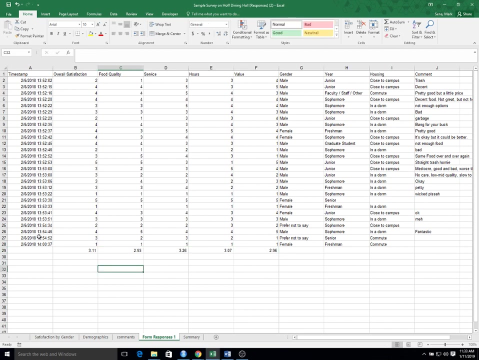 So this is just sort of a nuts and bolts. Um, and maybe that could go along with your demographics as well, Um. one last thing that I want to show you is called a correlation, So we don't need this figure anymore. 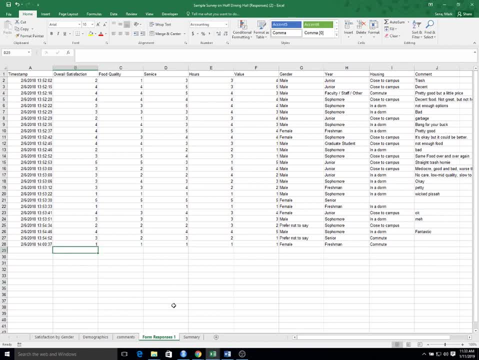 Um, so suppose that I want to uh understand what is driving this overall satisfaction. What's most important to um, if, if Hoff dining hall wanted to improve overall satisfaction, should they focus on the food quality, the service, the hours? 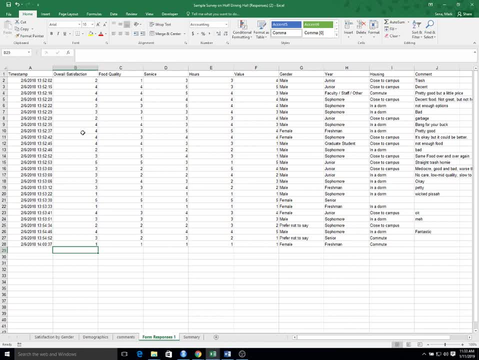 or the value, In order to determine that. I want to find out which one of these things is correlated with that. Um. so you might've done something like this in stat class, but there's a pretty simple function called actually. I'm going to put it over here. 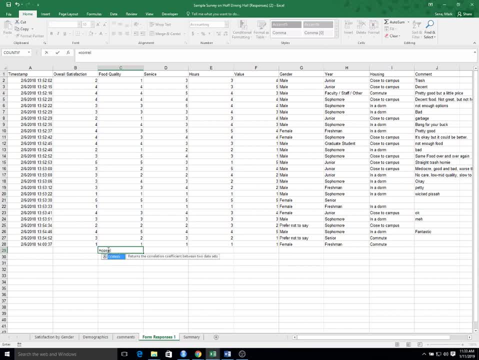 um equals corral, and I'm going to pick the satisfaction column. I'm actually going to absolute reference this range And the reason is because I want to be able to just paste over and I want to. so I want the correlation between food quality and satisfaction. 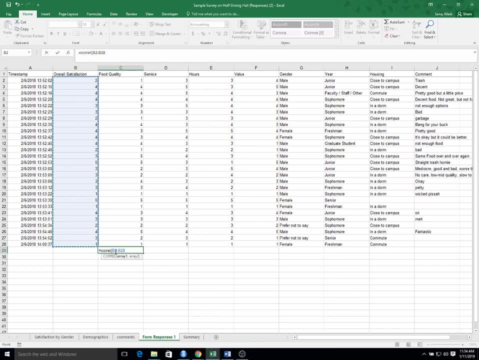 service and satisfaction, hours and satisfaction. So in order to do that, I want to freeze the range associated with overall satisfaction. So I'm going to click my F force here and then I'm going to put the comma and select the second range. 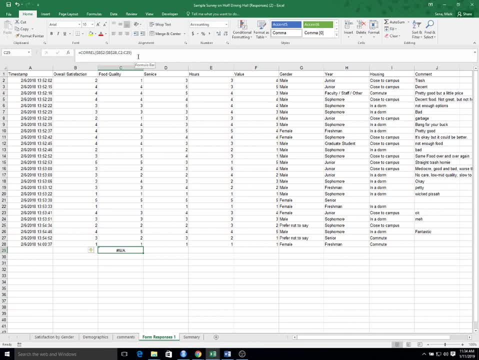 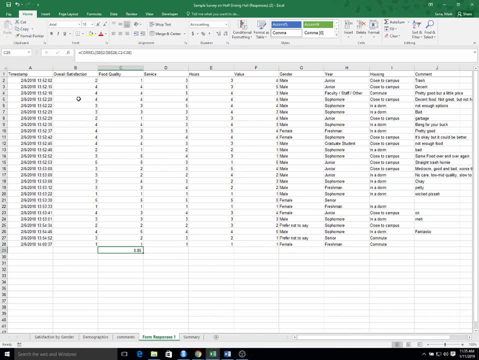 I scrolled down too far The uh. to do the correlation function, the number of rows has to be equal. So now that I have this first one done and there's actually a strong correlation there between food quality and overall satisfaction, I'm going to drag that over to the left, right to get the others. and now I'm 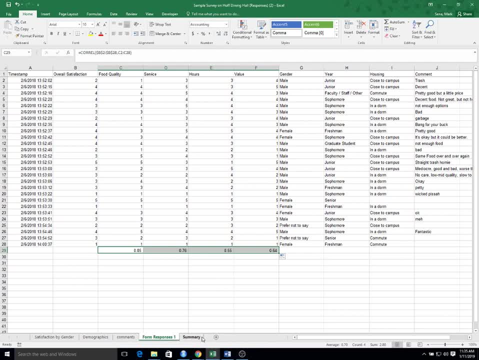 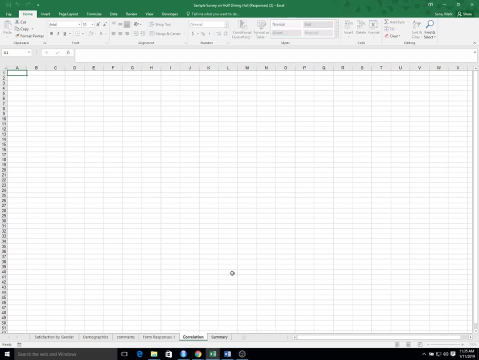 going to do something similar to what I did before. I'm going to start a new worksheet, which I'm going to call correlation, and I'm just going to copy over the data and move it around, just like I did before. so I'm going to copy these labels. 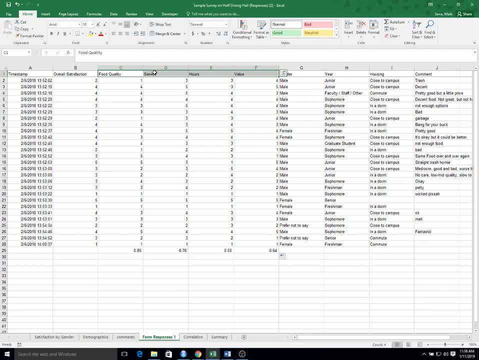 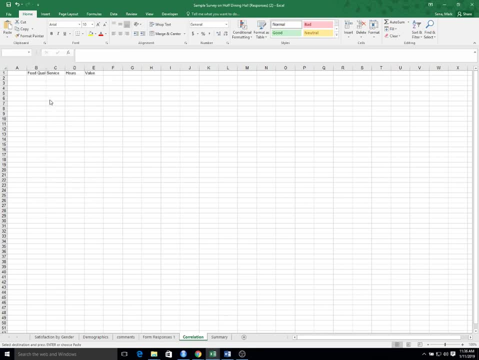 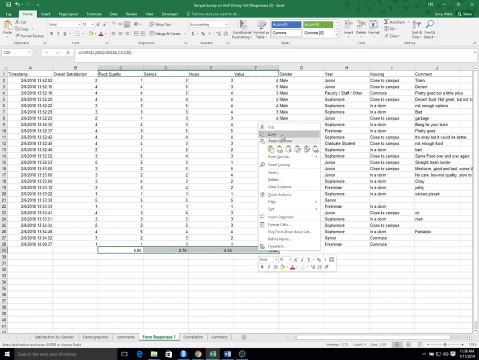 let me try that again. I'm going to start in row B, one this time, and then I'm going to copy the court, the values of the data, and then I'm going to copy the values of the data and then I'm going to copy the values of the correlation. 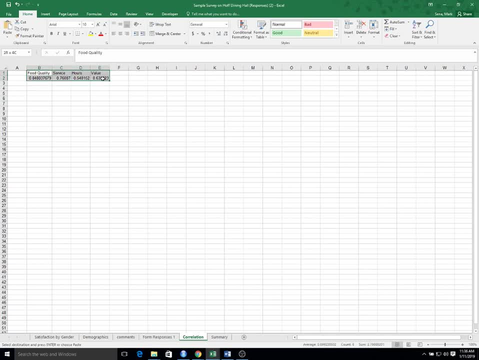 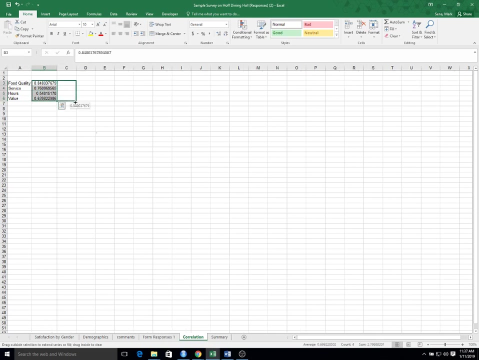 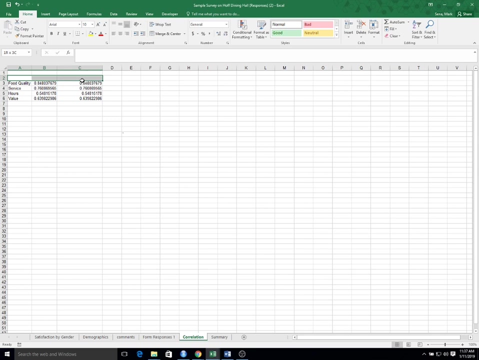 and then I'm going to copy and transpose these. you get rid of the original data and I'm actually going to make a second copy of that and I'm going to turn this into a little chart. I'm going to merge and center and call the heading correlation with. 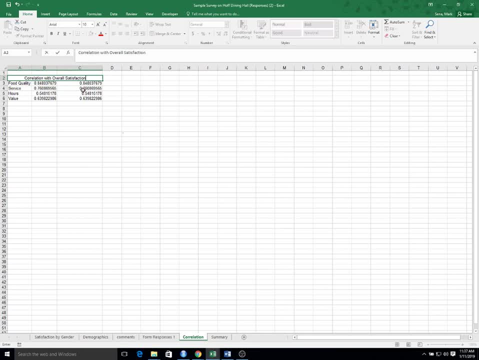 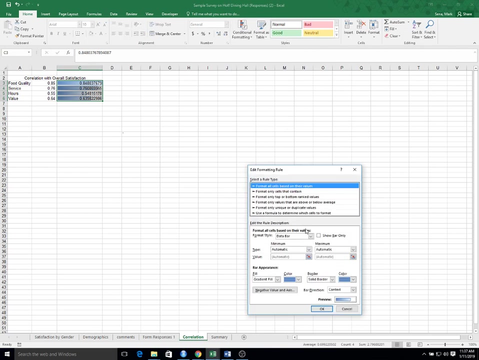 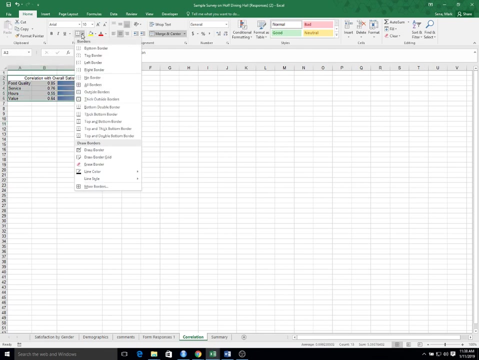 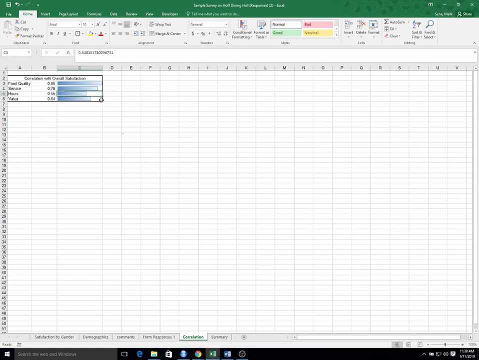 overall satisfaction. and this one I'm going to convert into a conditional format data bar and I'm going to go into the data bar. you, you And I'm going to edit it and I'm going to click on this option that says show bar only. So now I have this kind of cool little chart that shows my satisfaction in kind of a graphic. 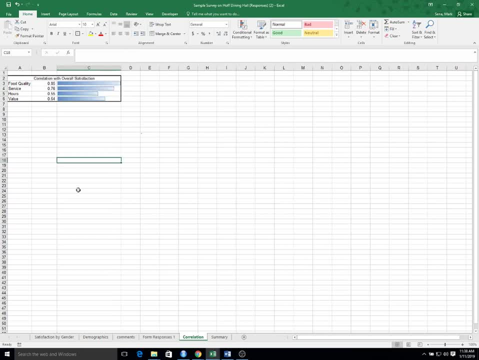 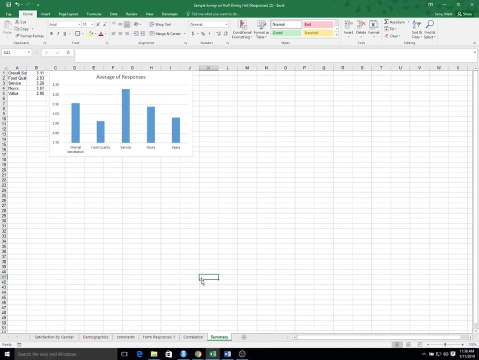 or format. So now we can see that food quality is the most important, followed by service hours and value Right, so that gives you an idea. again, your data is going to be different than mine, So there's going to be different things that you might have to do. 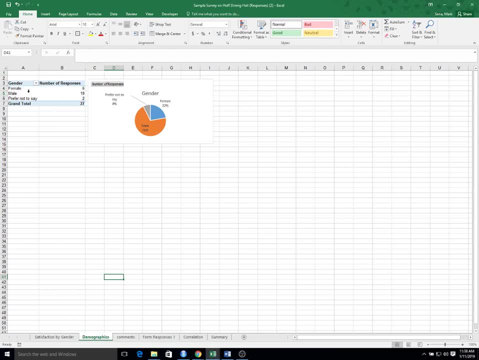 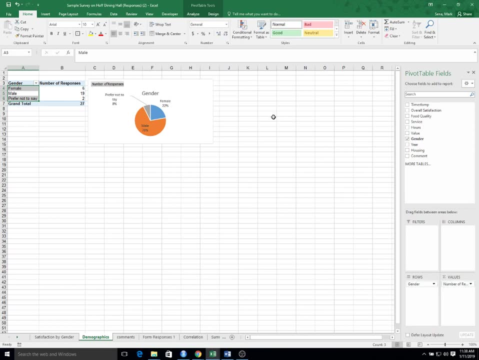 Some of you that have a lot of your data as text labels, You're going to need to do things that are similar to this. You might put some slicers in with it. So if you wanted, let's say I had like favorite shoe by gender and you had a multiple choice. 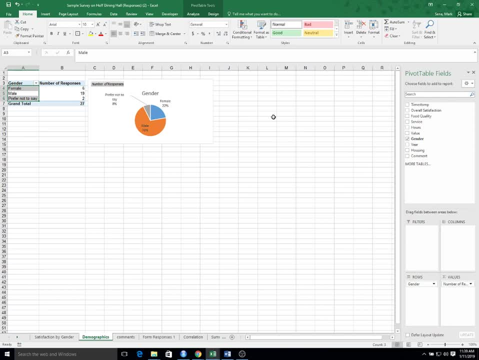 question. that was like Nike, Adidas, New Balance, Under Armour and you had data similar to this. You could set it up. You could set it up where favorite shoe is in the row and in the sum value, And then you could put a slicer for gender and then you could see what the percentage.